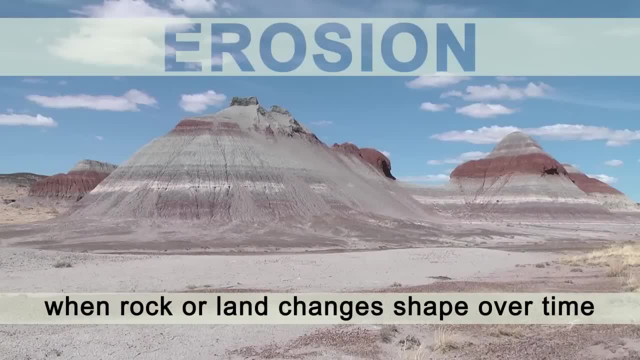 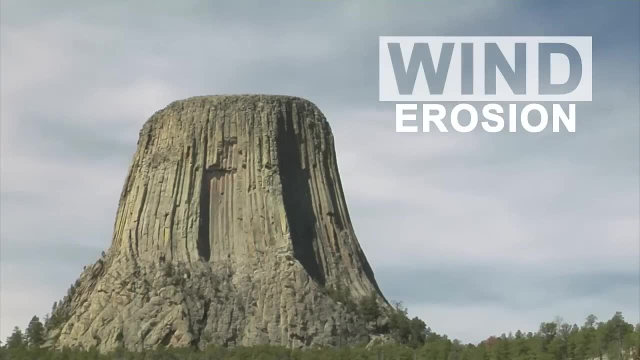 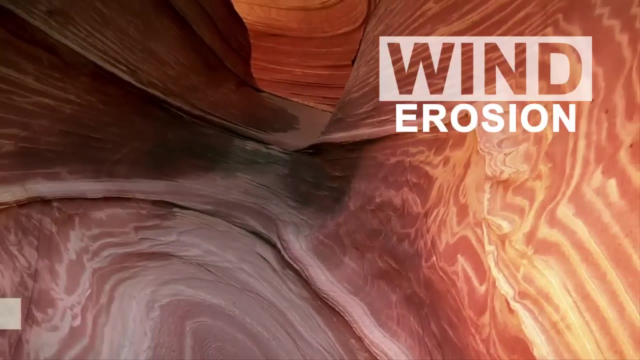 One such process is erosion. Erosion happens when rock or land changes shape over time. There are different types of erosion. One type is wind erosion. You may not think that wind can change the shape of Earth, but this has happened in many places. 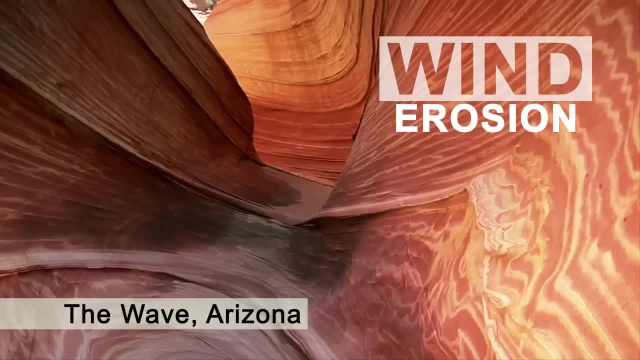 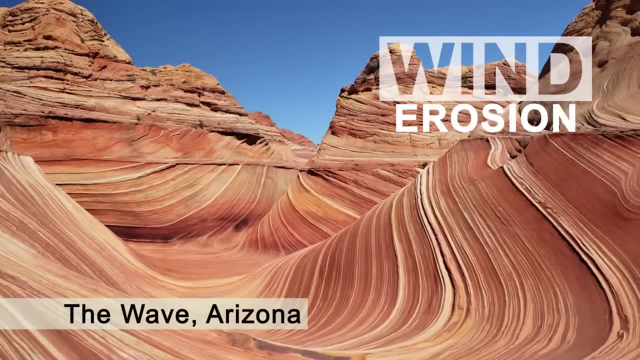 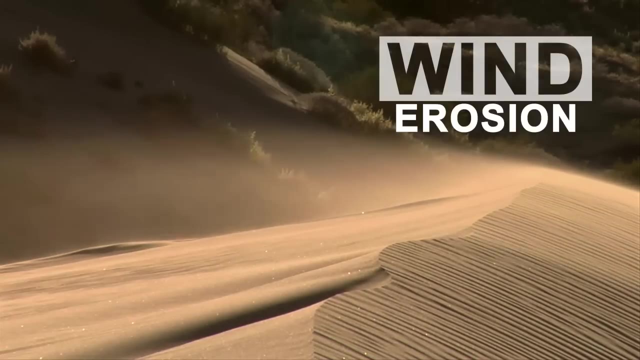 One location that has been shaped by wind erosion is in the southwest United States, in Arizona and Utah. This area is known as the wave because it looks like an ocean wave crashing. But how did it get this shape? Wind blowing through the desert carries sand along with it and blows across the rock. This 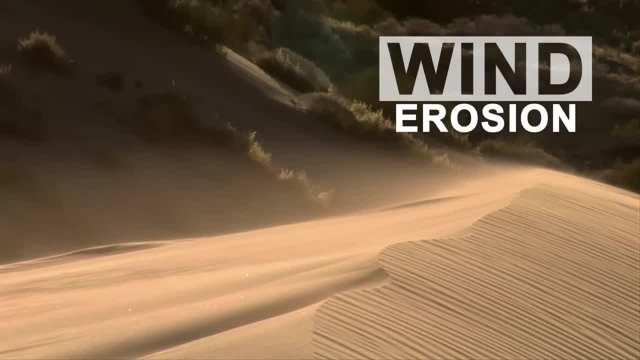 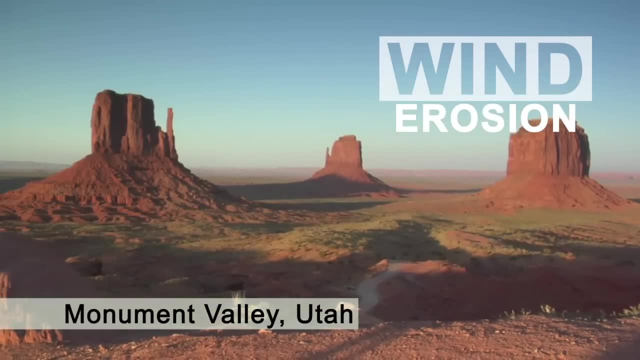 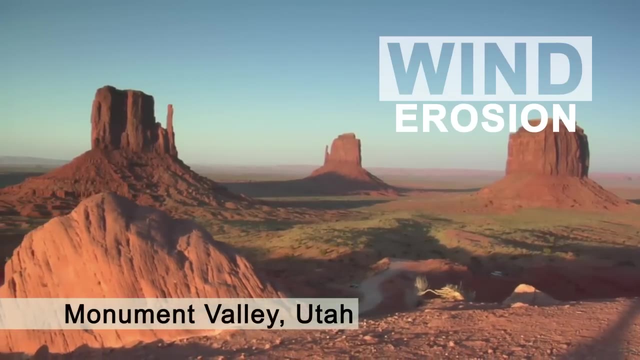 wears away small amounts of the softer rock and over a long enough time period, the wind creates unusual shapes in the rocks. This area of Utah called Monument Valley has some of these unusual rock formations caused by wind erosion. As the rock has been worn away, it has left behind tall, strong rocks. 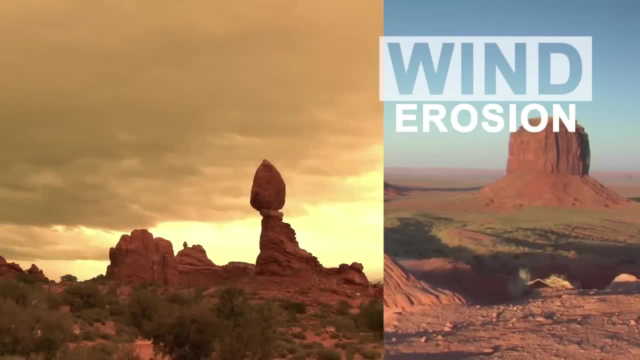 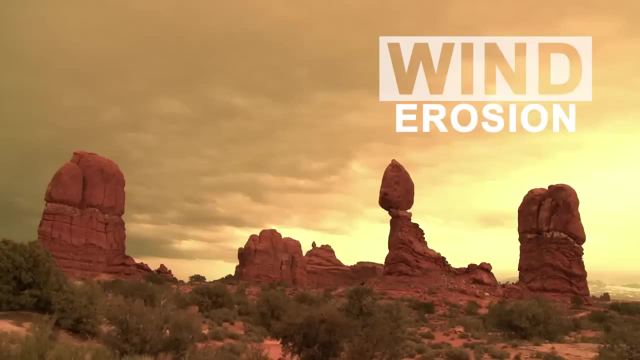 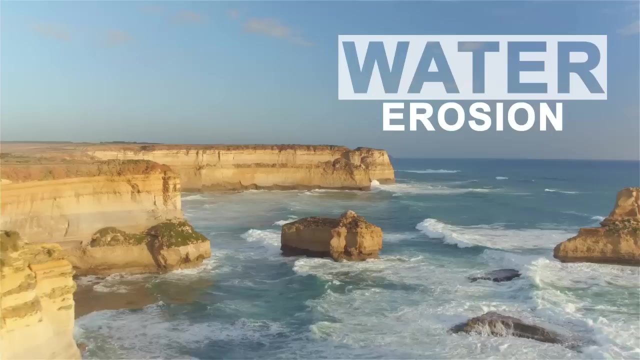 The rock is often found behind tall structures like these totem-shaped rock pillars. Wind erosion is common in areas of land that are higher in elevation, such as these formations, also in Utah. Another common type of erosion is water erosion. This occurs when water causes rock or land. 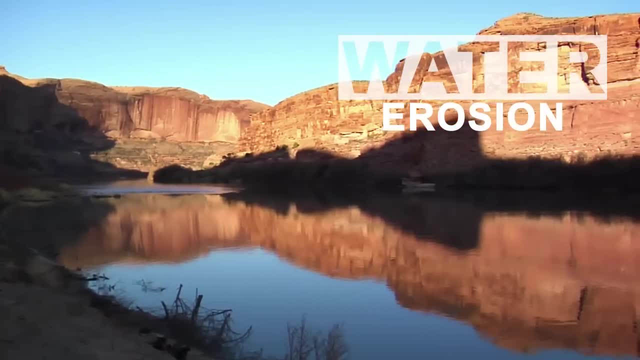 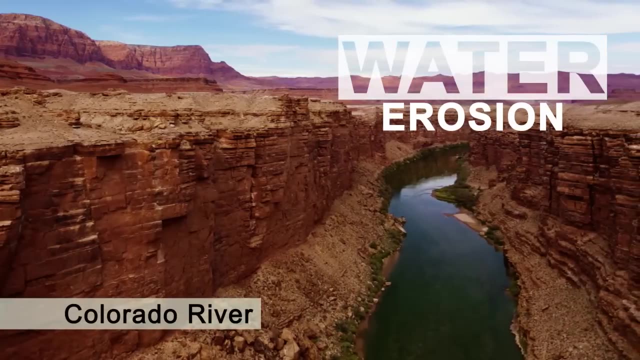 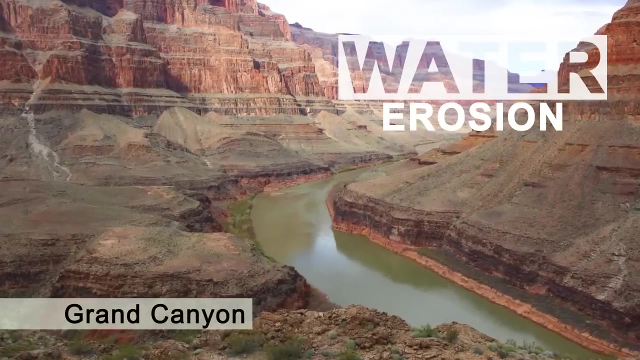 to change shape over time. One of the most dramatic examples of water erosion is also found in the United States. The Colorado River flows from Colorado to Mexico. Over millions of years, the water traveling this path created a canyon. This canyon is now called the Grand Canyon and is a well-known tourist attraction. 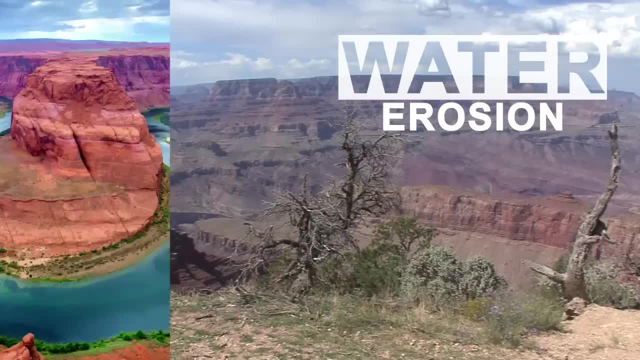 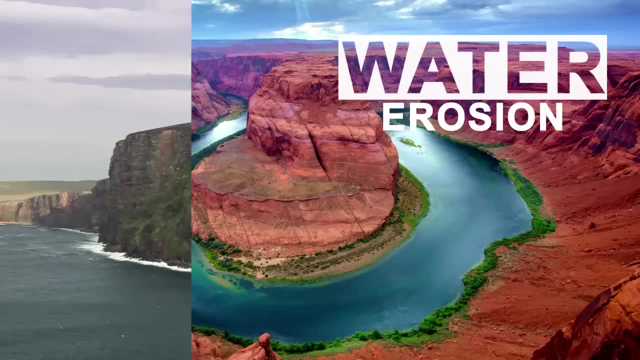 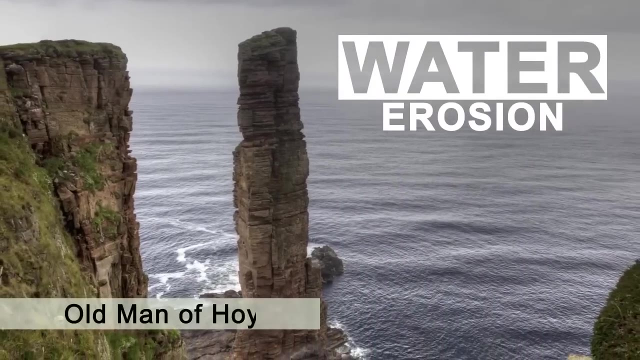 The canyon is a mile deep and up to 18 miles across at its widest areas. This amazing sight was shaped entirely by the water running over it day after day. Another amazing example of water erosion can be seen along the coast of Scotland, where you will find a rock formation known as the Old Man of Hoy. 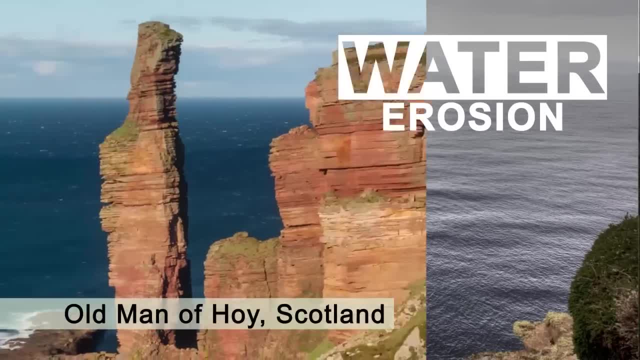 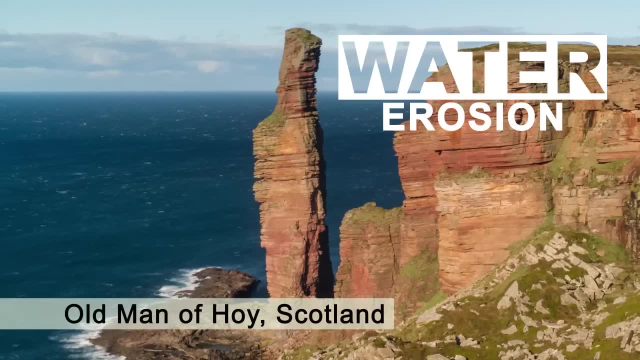 This rock formation is known as the Old Man of Hoy. This rock formation is known as the Old Man of Hoy. In the same way that river water can erode rock, ocean waves hitting the land again and again can also cause erosion. This particular formation is called a sea stack.